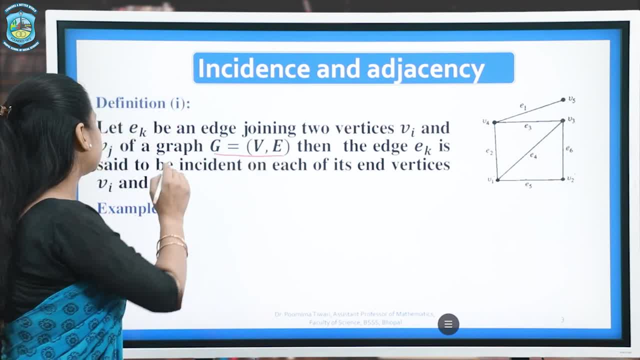 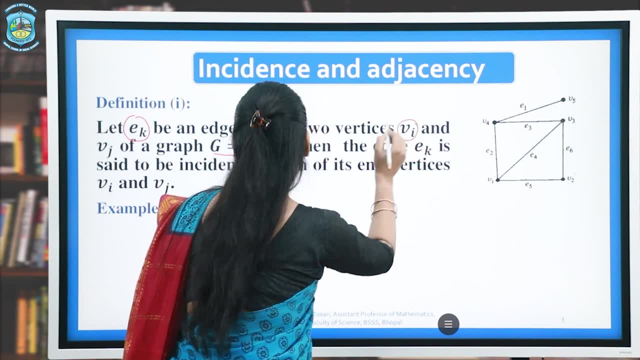 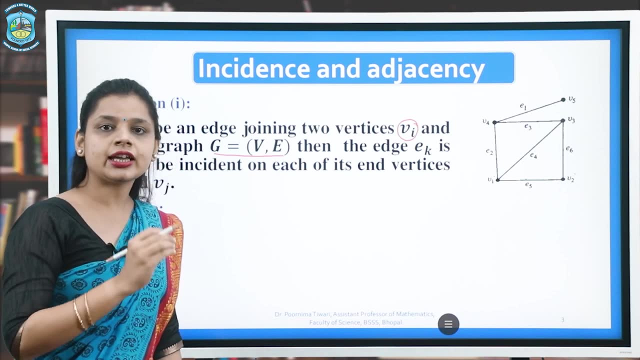 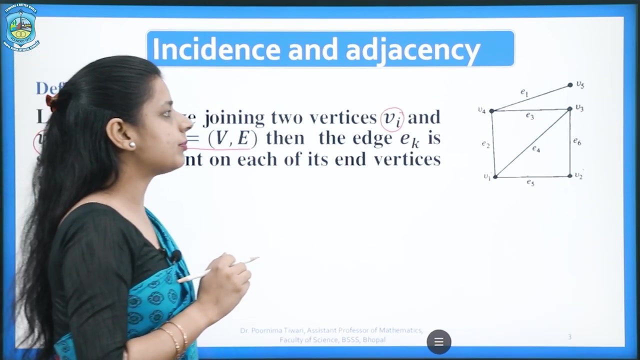 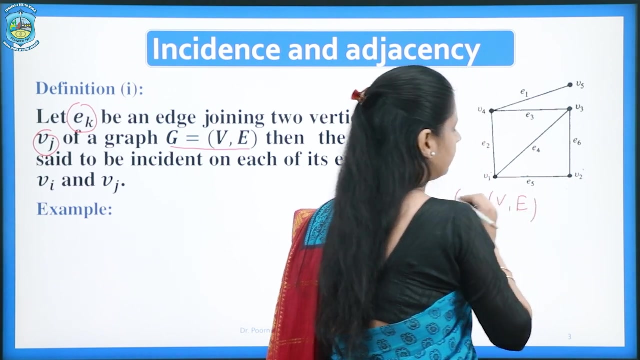 graph G is equal to VE and an age EK. This age EK joins two vertices, VI and VJ. Then we will say that this age EK is incident on its end vertices. For example, we consider this: graph G is equal to VE, where the set of vertices consisted. 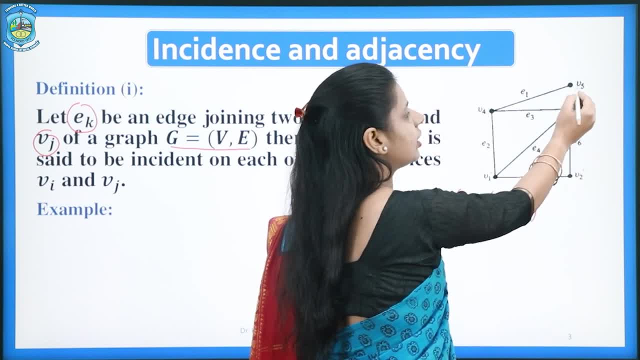 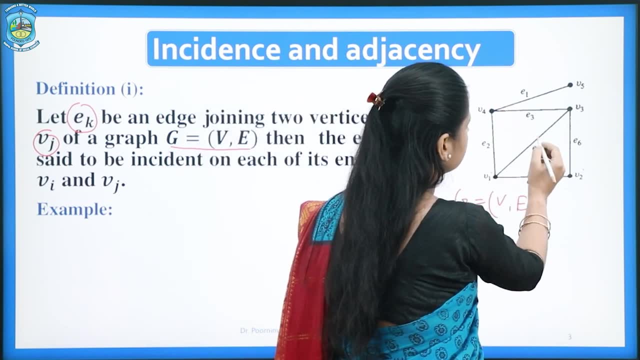 V1, V2, V3,, V4 and V5.. And set of ages consist E1, E2, E3, E4, E5 and E6.. Now let us consider the set of ages. For example, we consider this: graph G is equal. 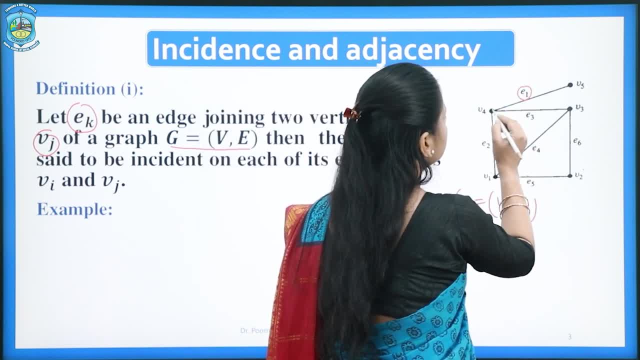 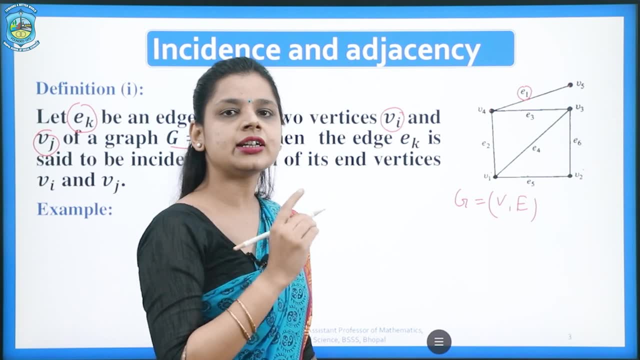 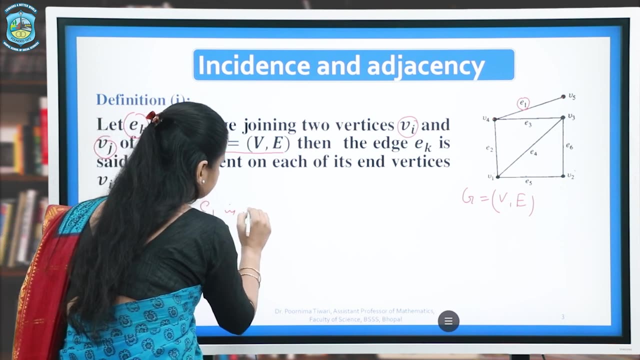 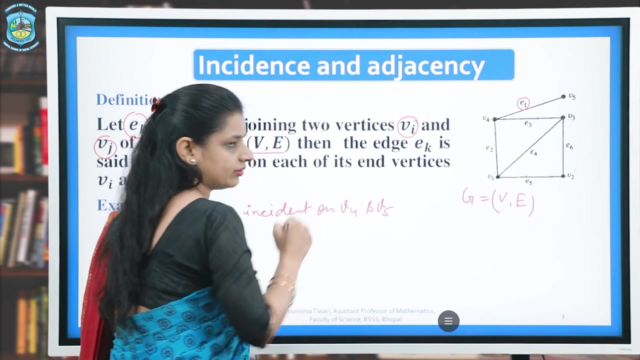 to V2,, E5,, E6, and E7, where the set of ages is K. So within the database the agency is the incident alterist of the sentences. so E1 is V4, V6, V5, and V7, V6. 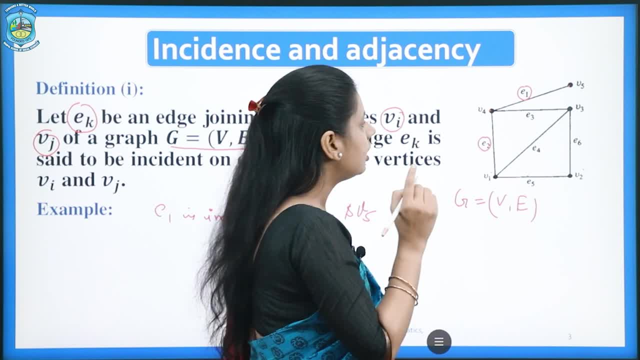 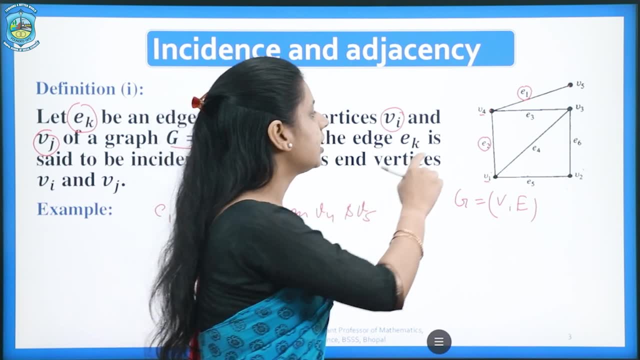 and V7. Then we will consider the chart. In the database, currency is the date, the time, the price time or the nation. In the database, the amongst sentences is the date. the E2 lies between the vertices V4 and V1. So we will call that E2 incident on V1 and V4. 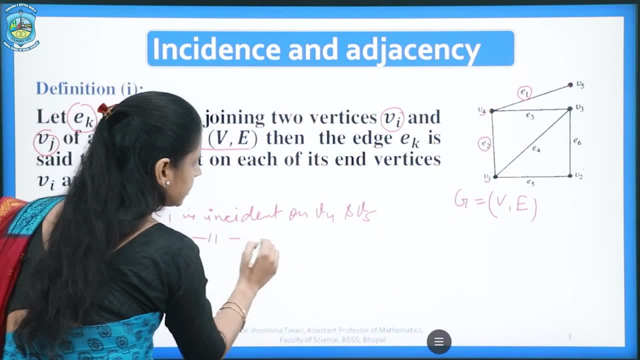 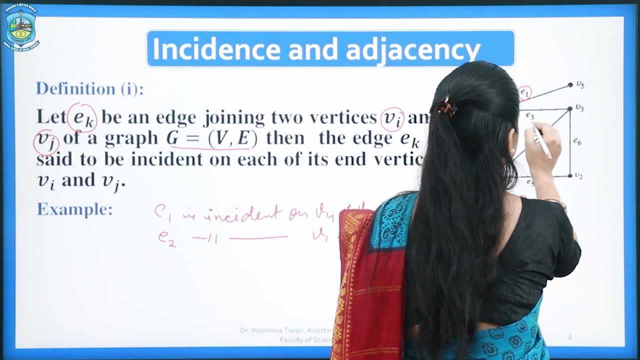 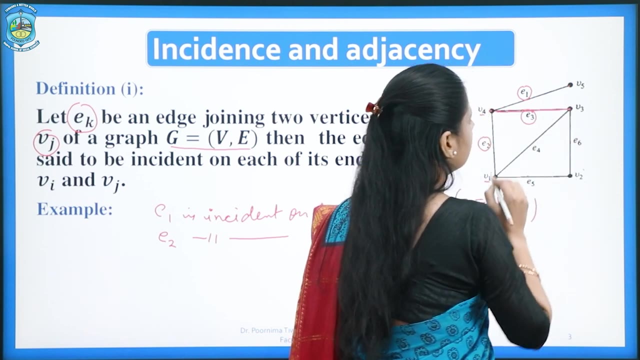 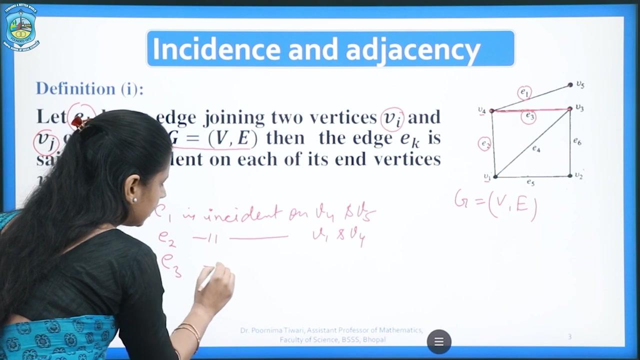 So second edge E2 is incident on V1 and V4.. Third edge E3, it join the vertices V4 and V3. So we will call that E3 incident on V3 and V4.. Edge E3 is incident on V3 and V4. 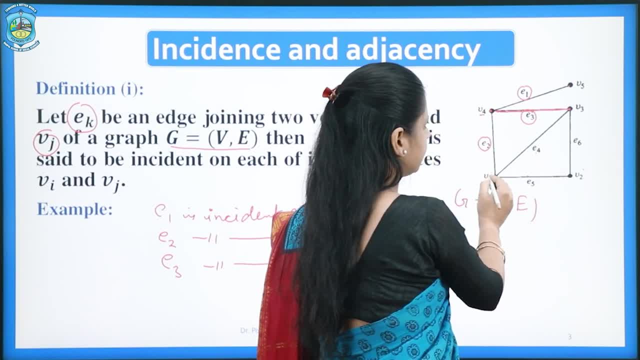 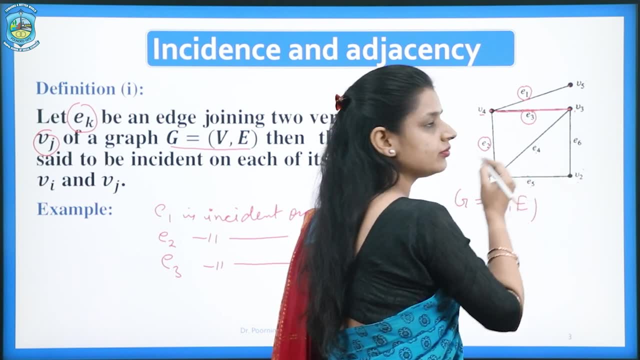 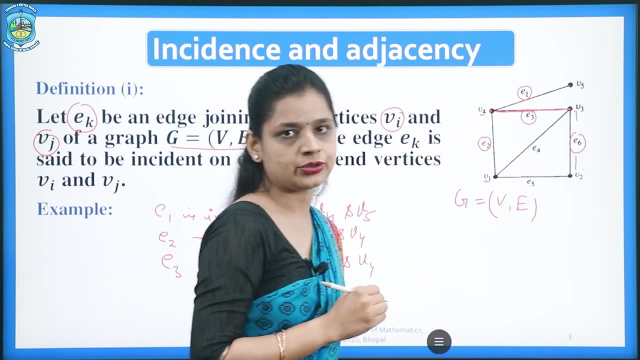 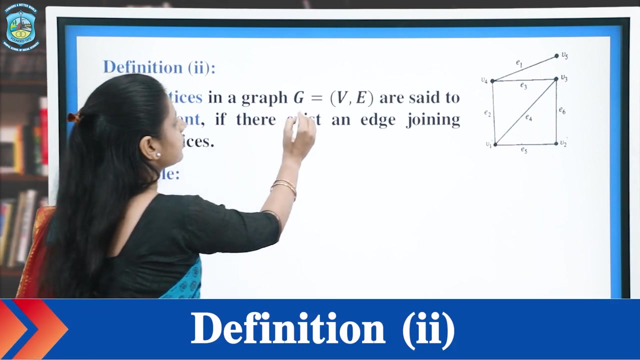 Likewise, edge E4 incident on V1 and V3, edge E5 incident on V1 and V2 and edge E6 incident on V3 and V4.. v2.. Second definition is about adjacent vertices. Two vertices of this graph g is equal to ve. 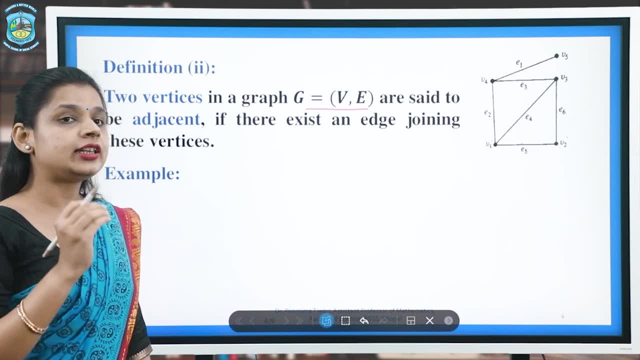 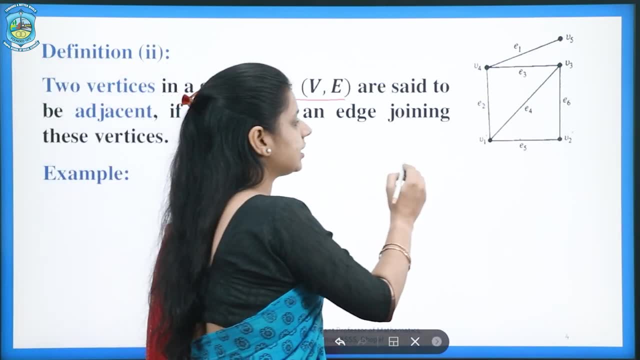 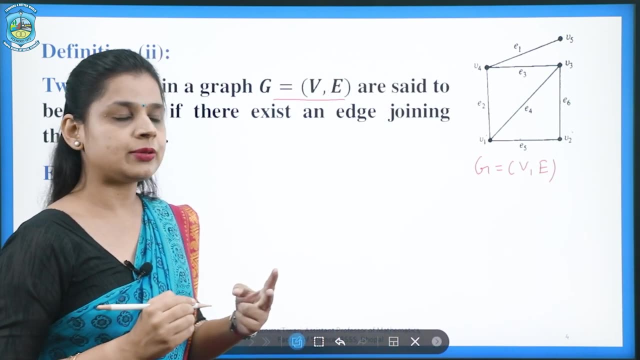 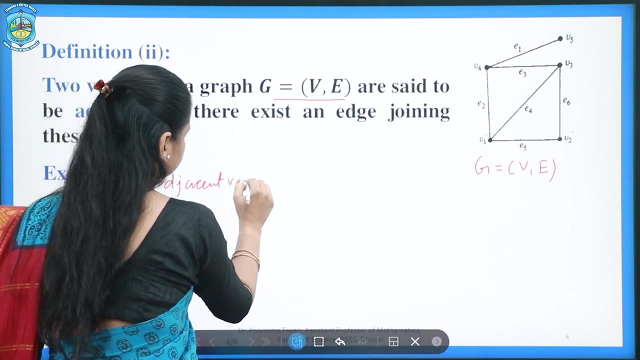 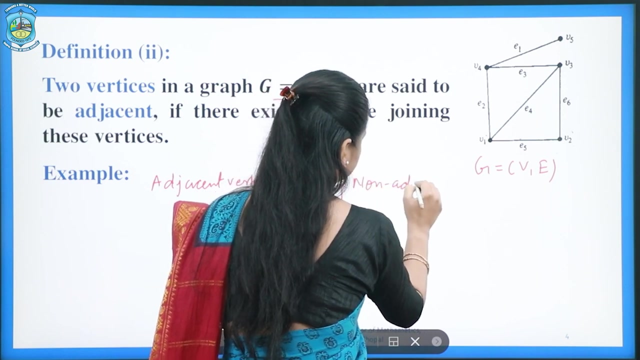 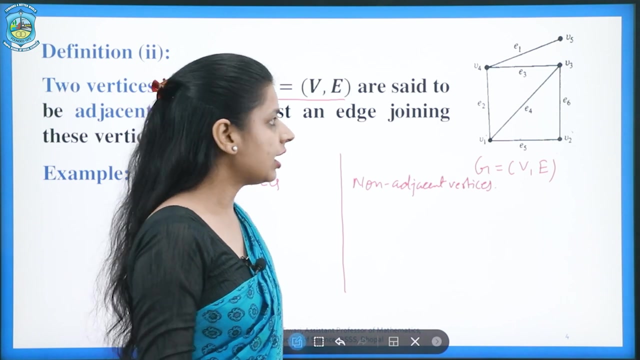 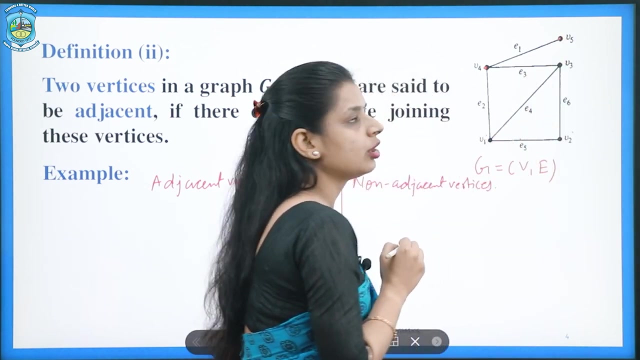 are called adjacent if there exists an edge joining these vertices. In the example we will consider the previous graph, g is equal to ve and we will find two types of vertices: one is adjacent vertices and the another one is non-adjacent vertices, As, per definition, we find that this V4 and V5 joins by edge e1.. 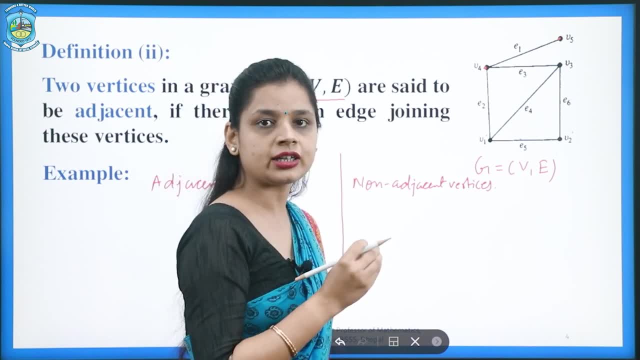 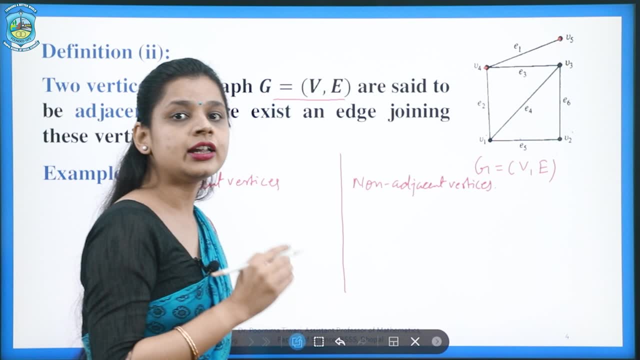 So there are two tight or solid points, g and gt, but our product can be avoided. in the next step, where gt is very much directed towards one logo is age E1 in between the vertices V4 and V5. So vertices V4 and V5 are adjacent vertices. 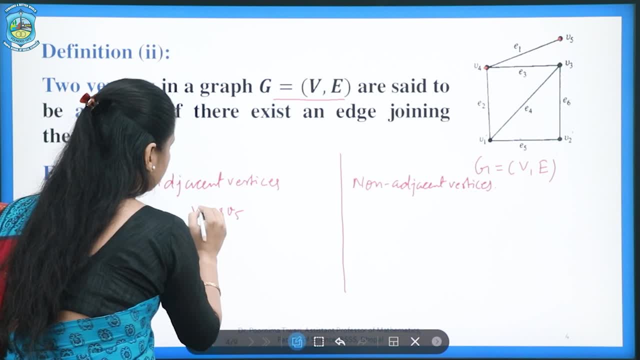 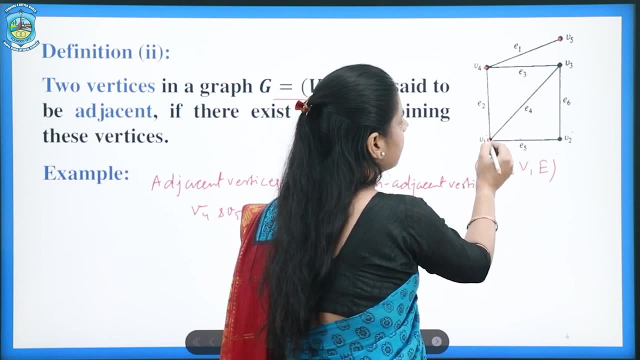 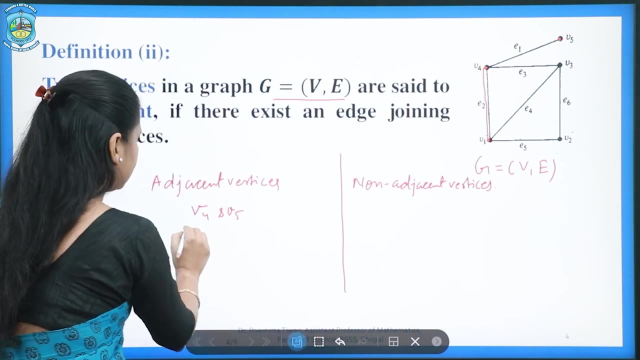 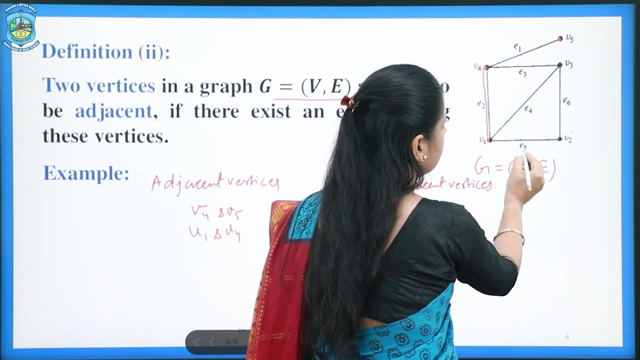 So this pair, V4 and V5, is adjacent vertices. Now see, there is an age E2 in between the vertices V1 and V4.. So V1 and V4 are adjacent vertices. Similarly, there is age E5 between V1 and V2.. 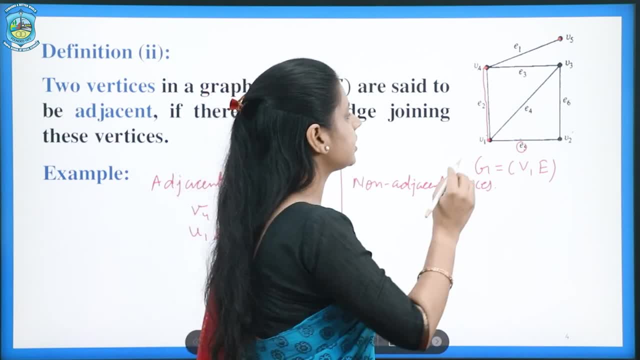 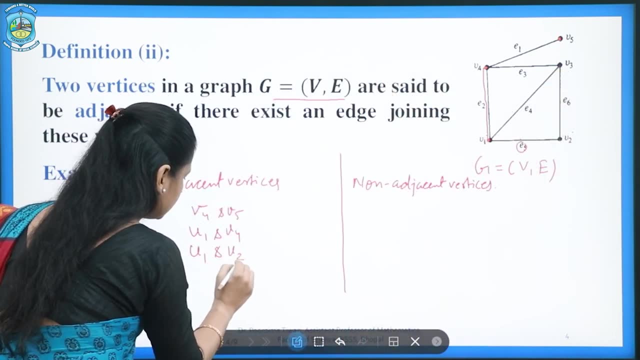 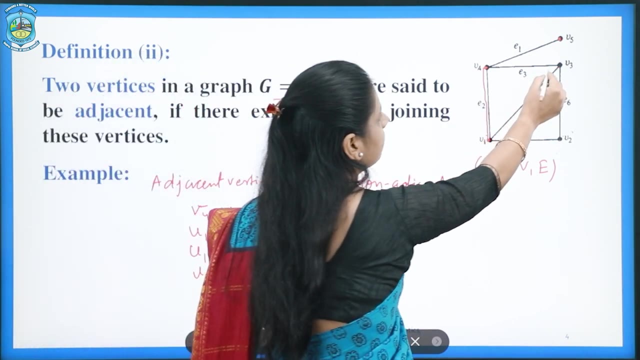 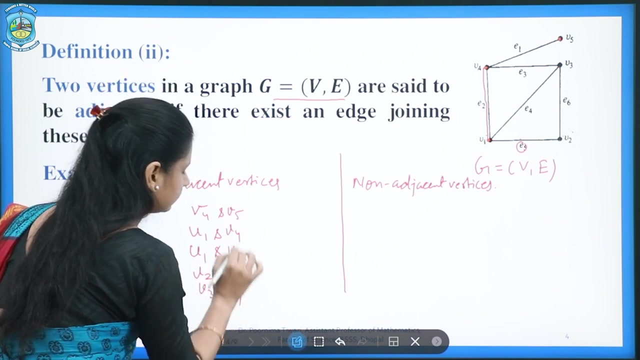 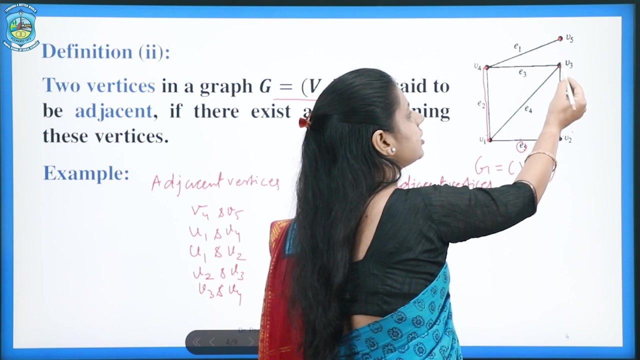 So V1 and V2 are adjacent vertices. V2 and V3 are adjacent vertices. So V1 and V2, V2 and V3.. Likewise, V3 and V4 are adjacent vertices. Now we see that there is no age joining these. 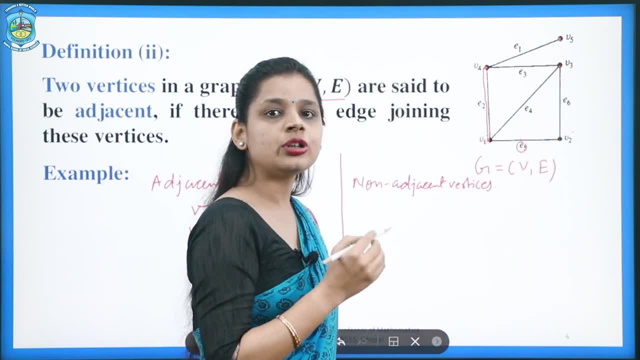 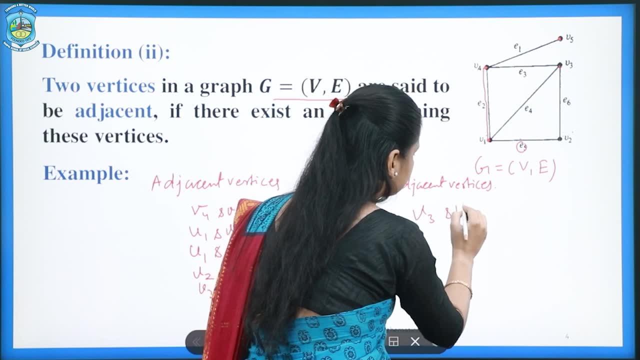 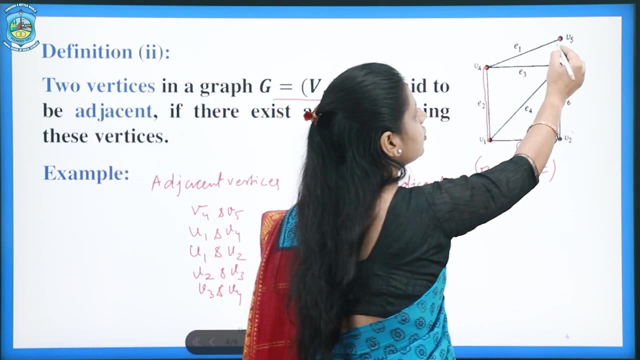 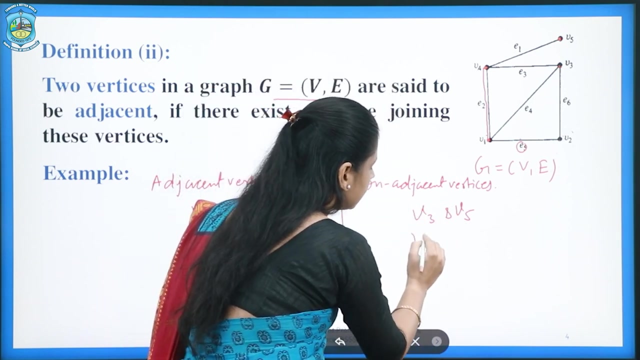 two vertices: V3 and V5. So they are non-adjacent vertices. So this pair, V3 and V5, are non-adjacent vertices. Next, we see that there is no age joining the vertices V2 and V5. So this pair, V2 and V5, is. 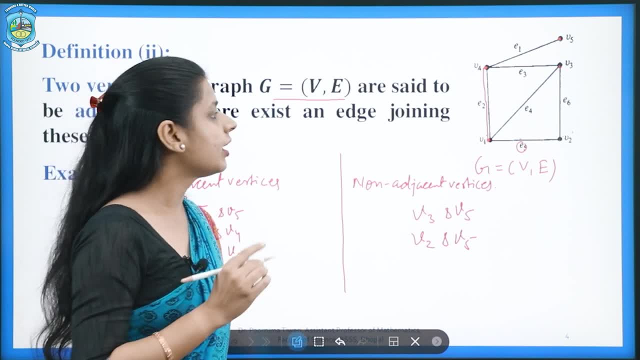 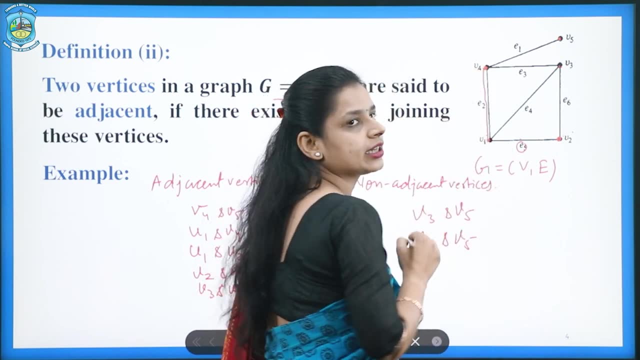 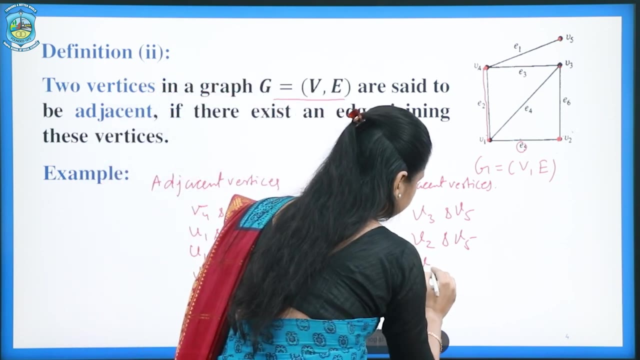 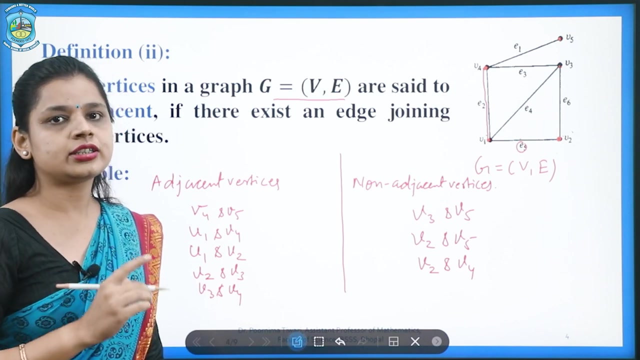 non-adjacent vertices. Next we see that there is no age joining this vertex V2 and this vertex V4.. So V2 and V4 are non-adjacent vertices. So in the graph we find adjacent and non-adjacent vertices. 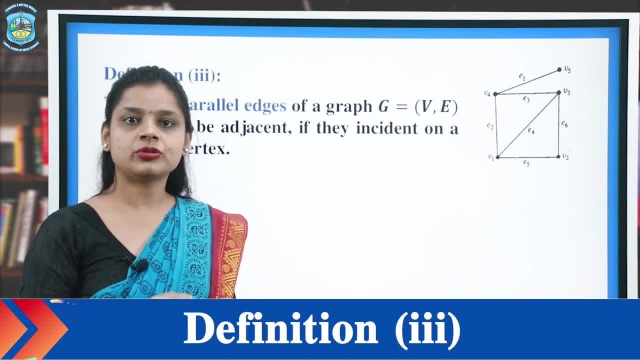 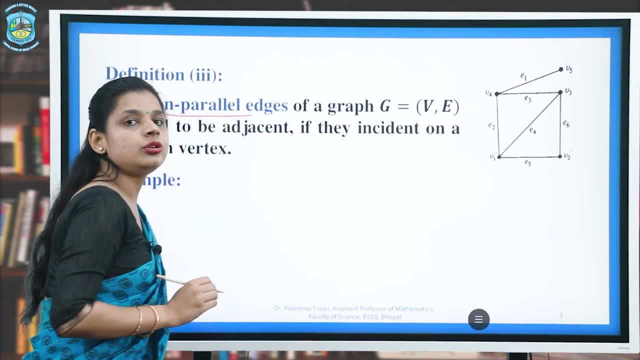 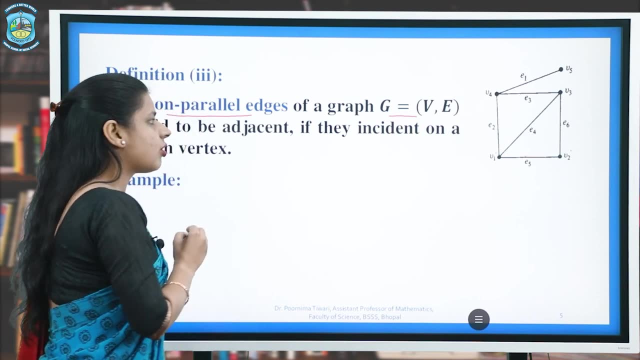 Third definition is about adjacent ages And you must note it down. This concept is defined only for non-parallel ages. So two non-parallel ages of any graph G are called adjacent if they are non-adjacent. So if they are non-adjacent, then they are non-adjacent, So if they are. 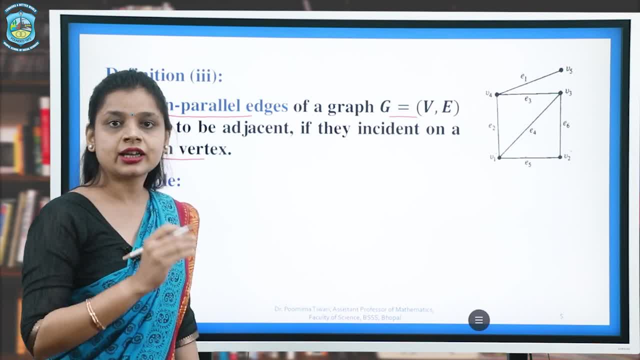 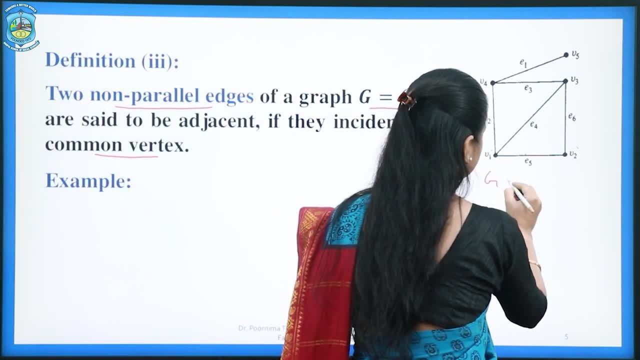 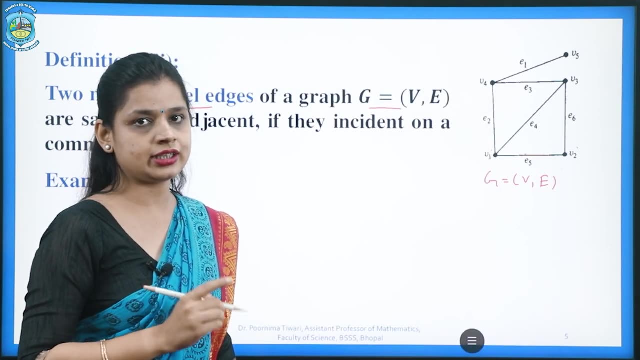 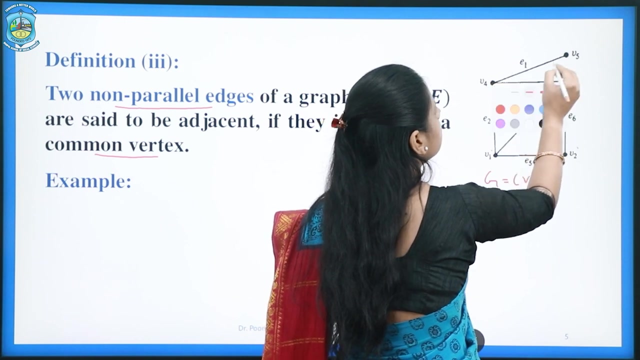 non-adjacent or fr parental. it doesn't apply. that simply So loose baruPutin works in this case Similarly for non-adjacent ages of any graph. these inch value erssembles in links up to the final cluster we want to follow. Height quantity and his radial douligare are dish. 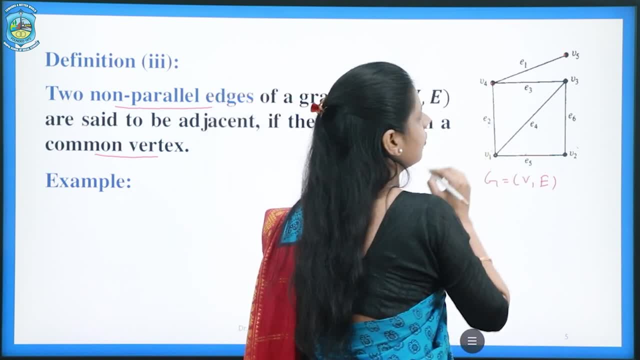 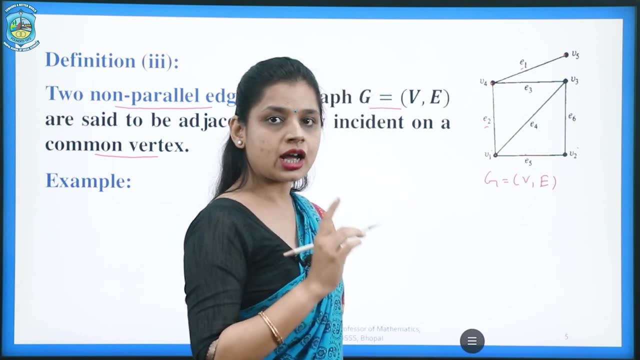 Incident on all edges: Hi. The wI by m existence is equal to the common vertex number And for both occurrences, edge E2. incident on V4 and V1.. That is edge E1 and E2 incident on a common vertex, V4.. 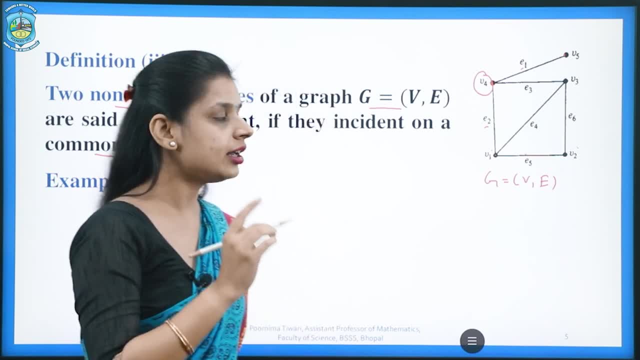 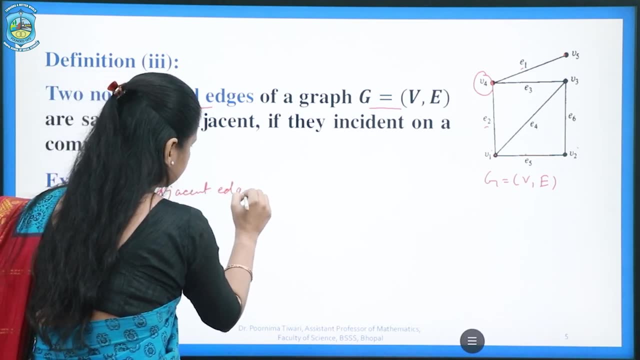 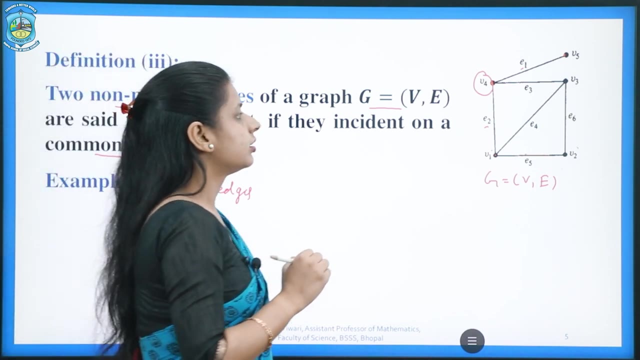 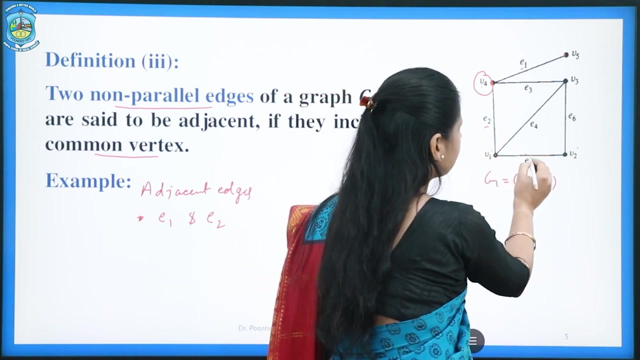 So the edges E1 and E2 are adjacent edges. So if we talk about adjacent edges, So first pair is E1 and E2.. Now just see E2 incident on V4 and V1 edge. E5 incident on V1. 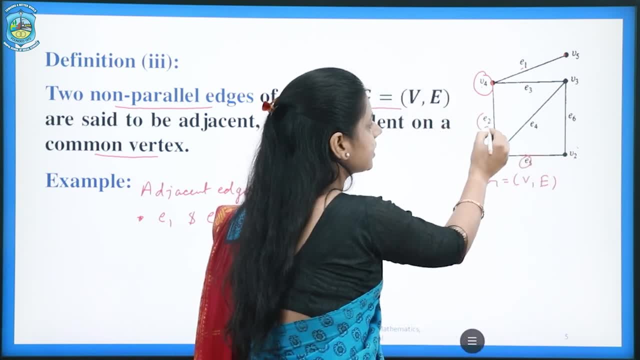 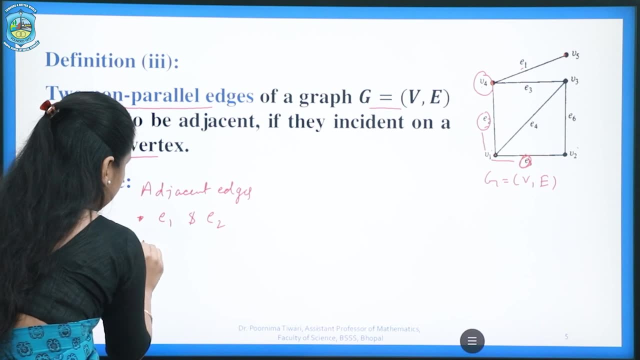 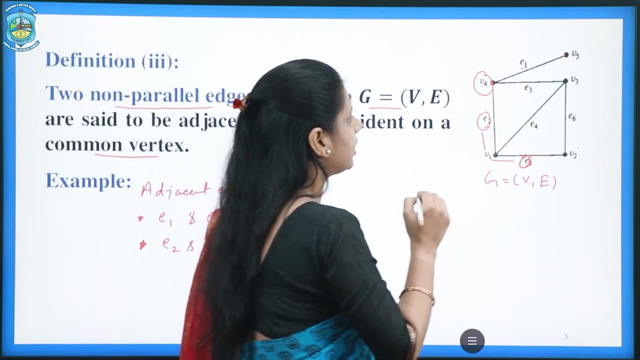 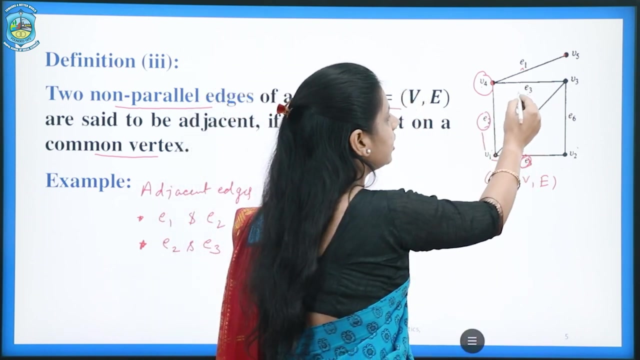 and V2.. That is, the edges E2 and E3 have this common vertex V1. So the edges E2 and E3 are adjacent edges edges. Likewise we can find the A1, E1 and E3 are adjacent edges. E3 and E4 are adjacent. 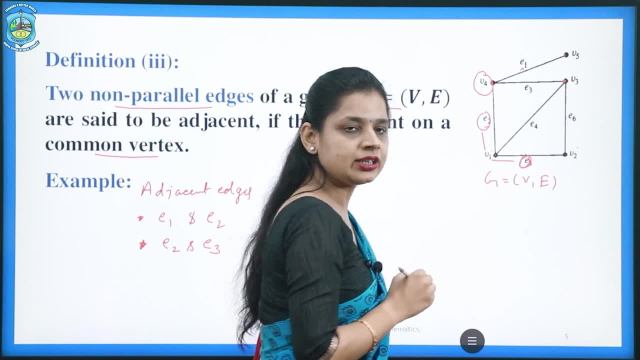 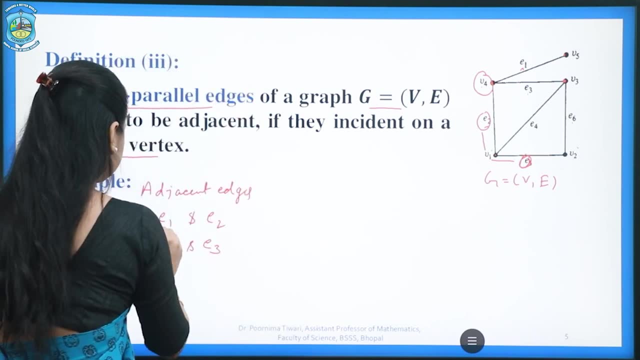 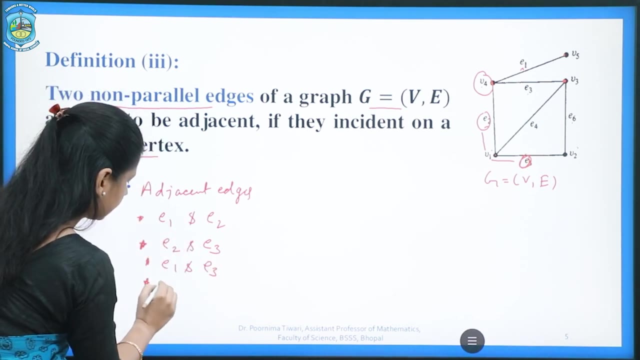 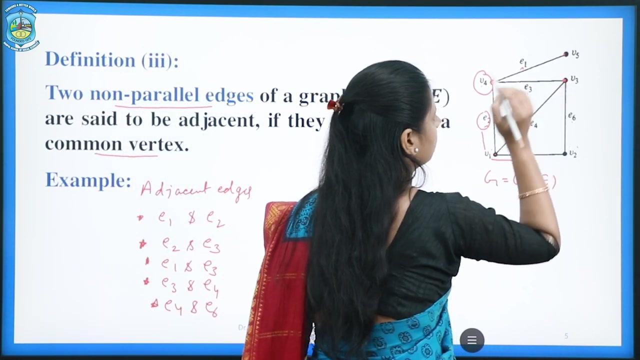 edges because they have this common vertex: V3.. E3 and E6 are adjacent edges. So what? we find? that E1 and E3 are adjacent edges. E3 and E4 are adjacent edges. E4 and E6 are adjacent edges. Both have one common vertex: V3.. Likewise we can find another pairs too. 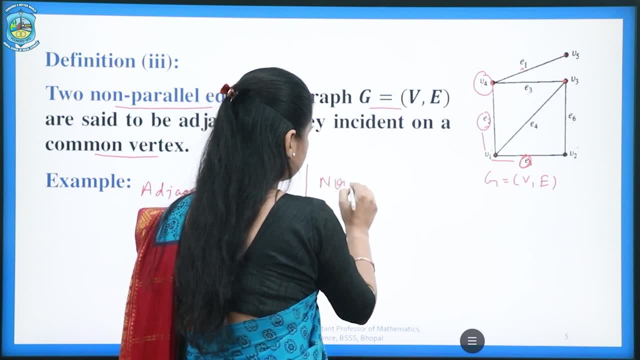 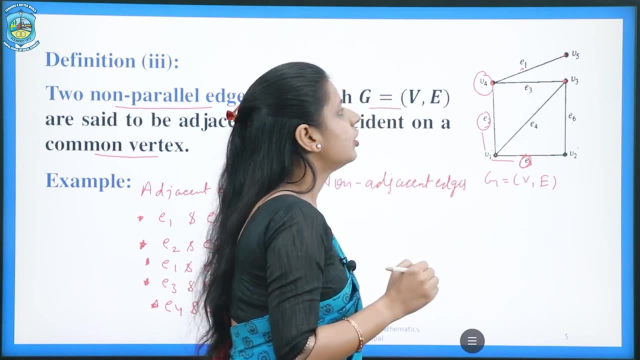 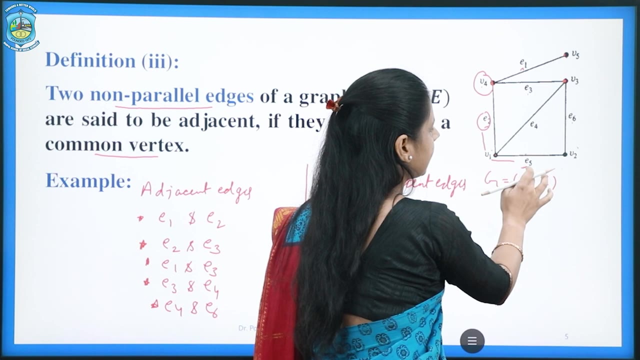 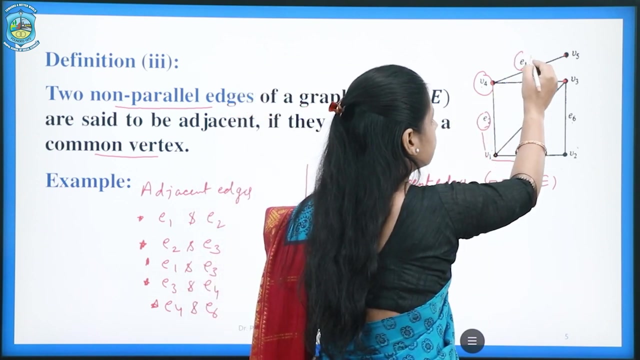 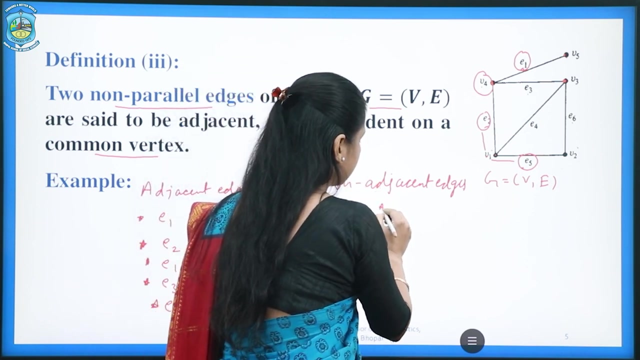 Now if we talk about E1 and E6. non-adjacent edges. So see this edge E1 incident on V4 and V5 and this edge E5 incident on V1 and V2.. So in between the edges E1 and E5 there is no common vertex. So this pair E1 and E5 is 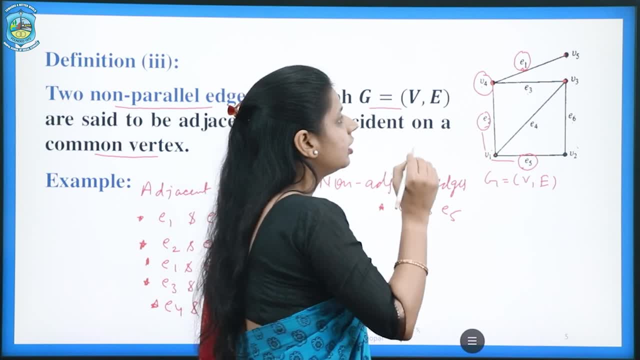 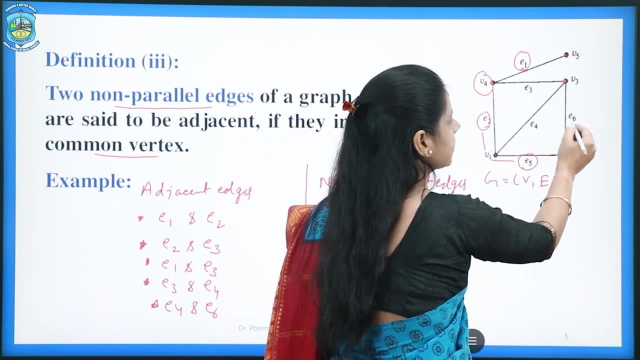 non-adjacent edges. Similarly, E1 lies between vertex V4 and V5, E6 lies between the vertex V3 and V4. So there is no common vertex E1 and E5. So this pair, E1 and E5, is non-adjacent edges. 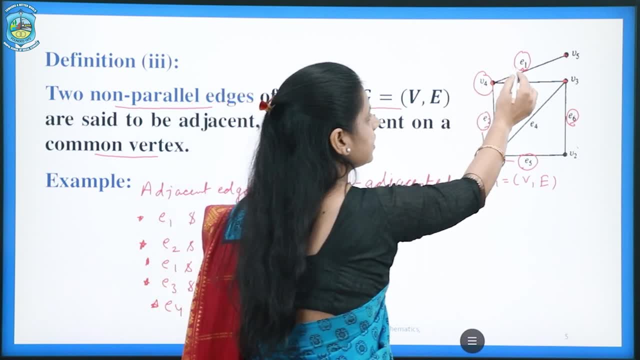 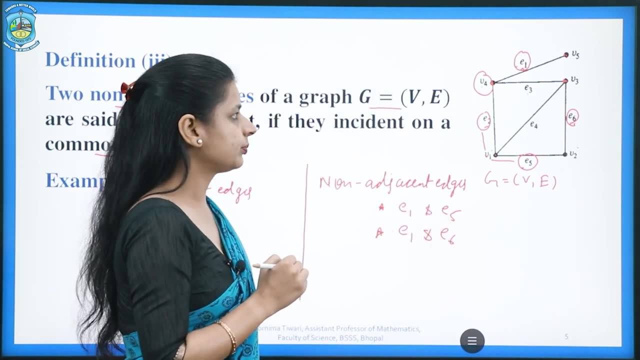 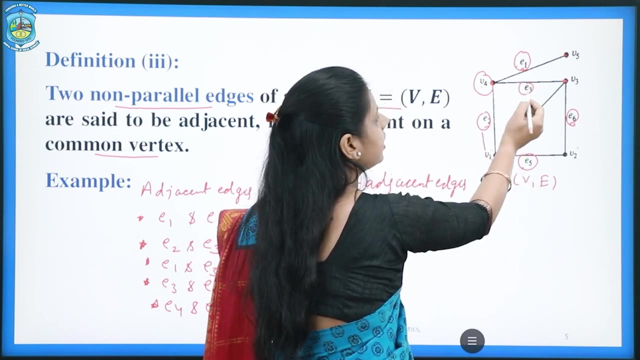 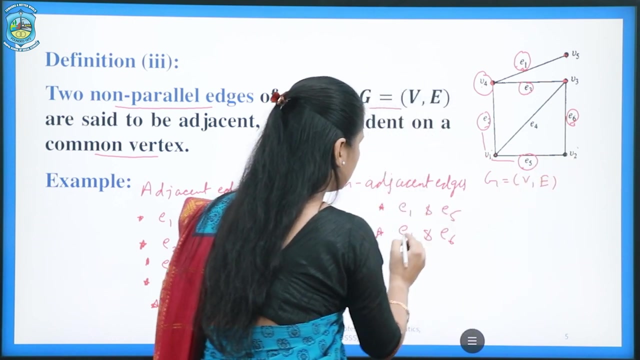 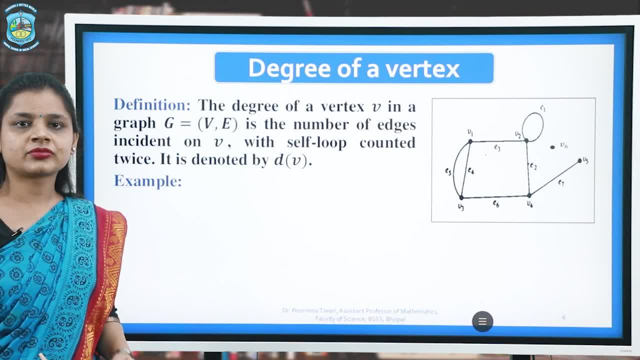 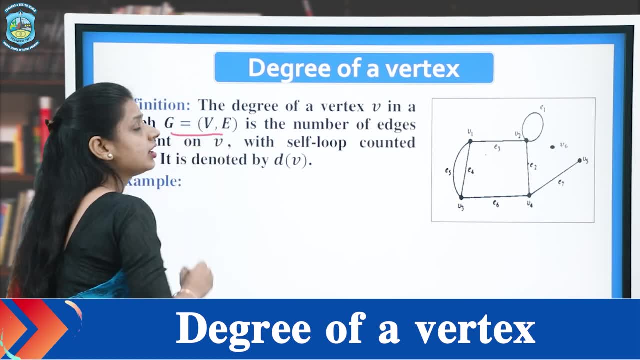 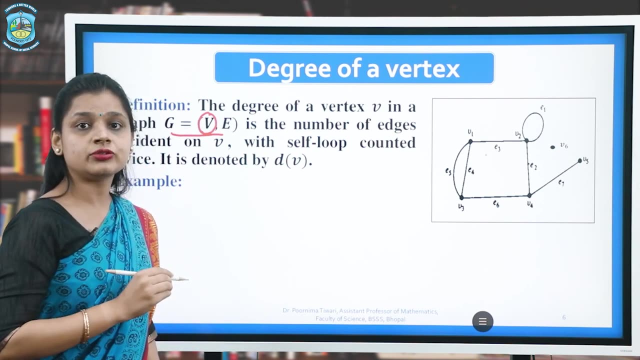 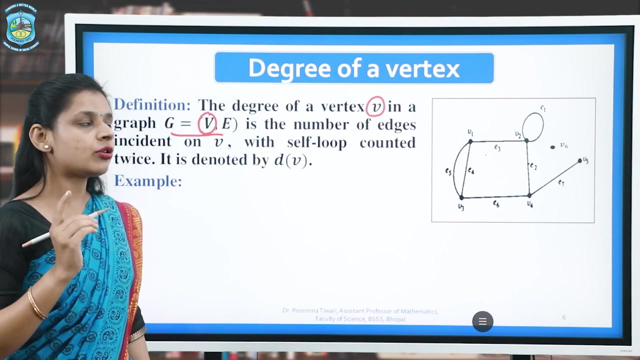 you may find another pairs too. Next concept is degree of a vertex. We have to consider a graph and we can find degree of each element of this set of vertices which is known as vertex. So the degree of vertex V is the number of edges incident on V1 and E5.. So 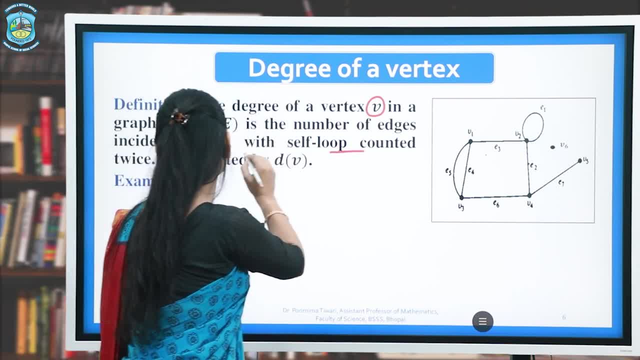 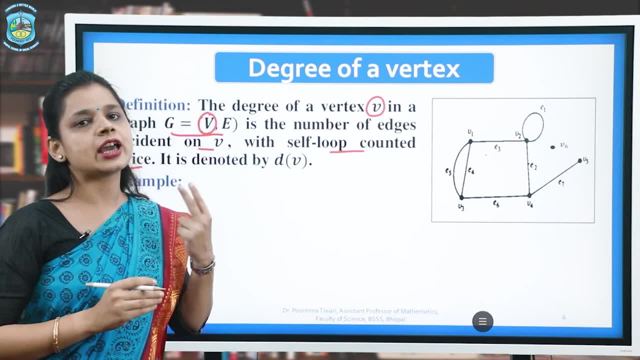 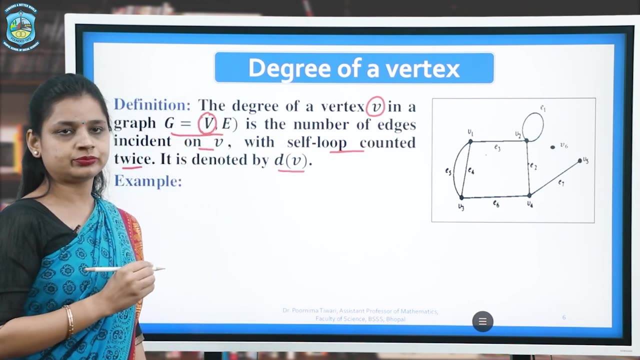 V1 and E5 are not totally identical, So in this case we have to consider a vertex that is smaller than V2 and V3, with self-loop counted twice. You must note down that is in the case of degree for the self-loop we have to count to. degree of vertex is denoted. 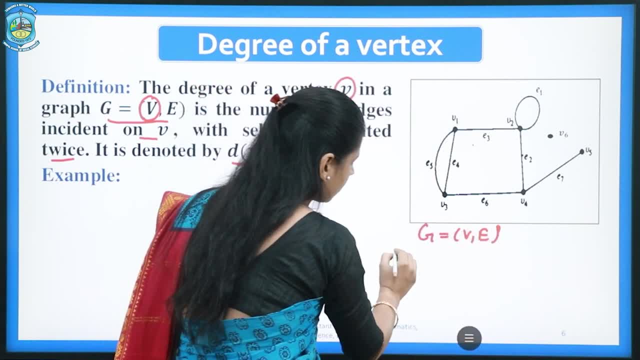 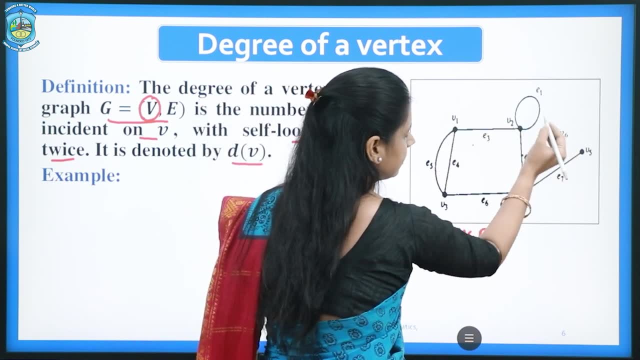 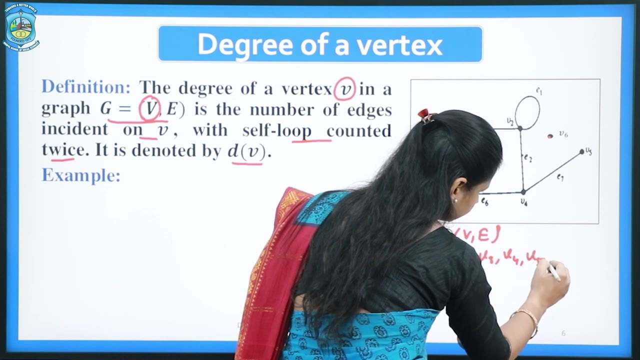 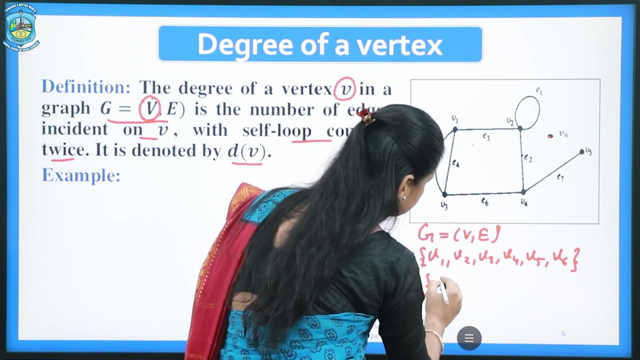 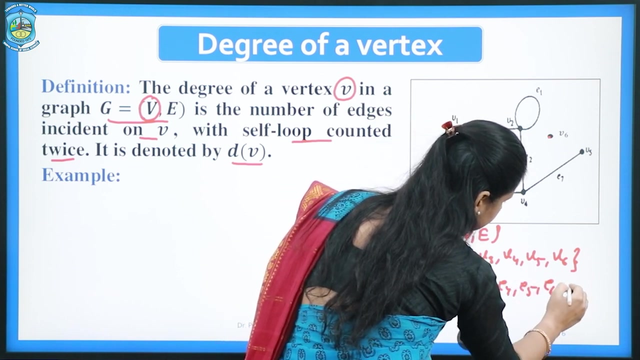 by D of V. for the example, we consider this: graph G is equal to VE, where the set of vertices V1, V2,, V3,, V4,, V5 and V6 and set of edges as the elements E1, E2, E3, E4, E5, E6, E7. 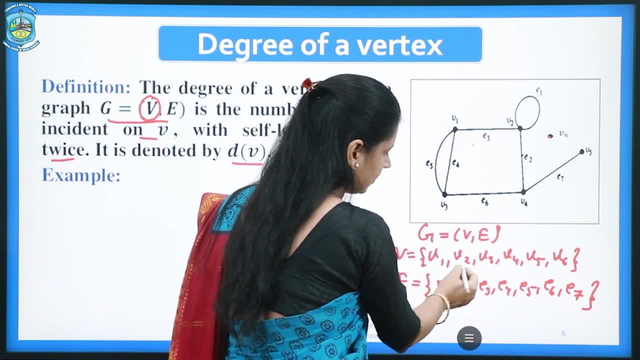 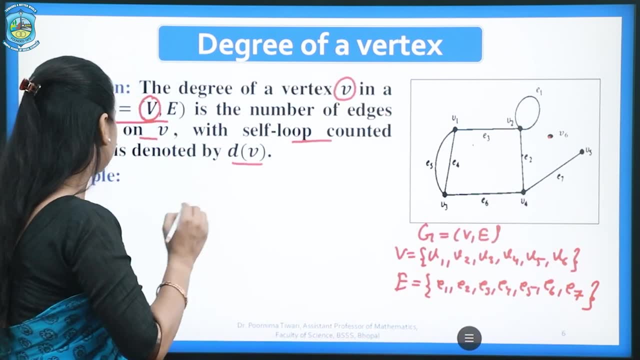 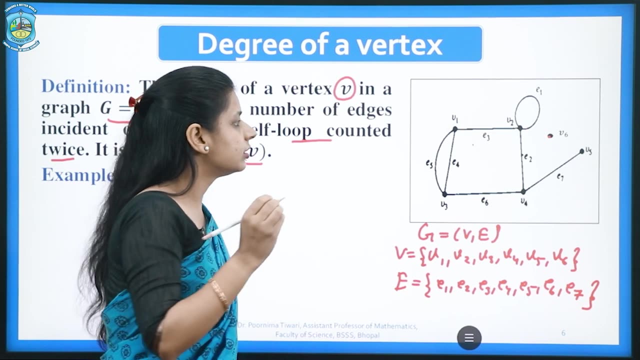 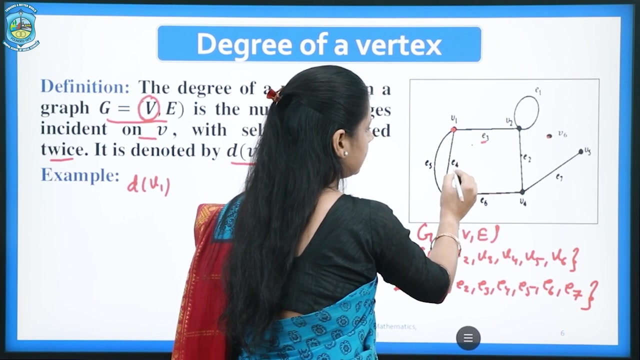 and we may find degree of each vertex: V1, V2, V3, V4,, V5 and V6.. Degree of V1 is the number of edges incident on V1.. So we see that on this vertex, V1, three edges incident: E3, E4 and E5. 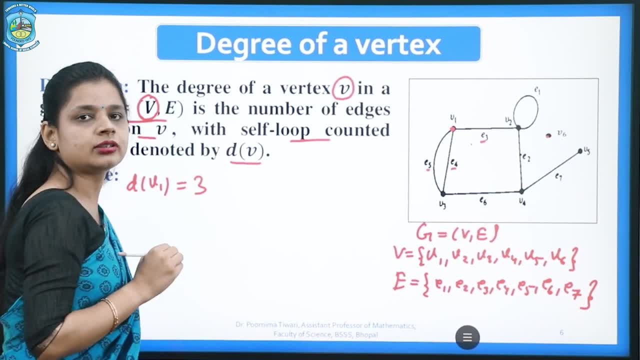 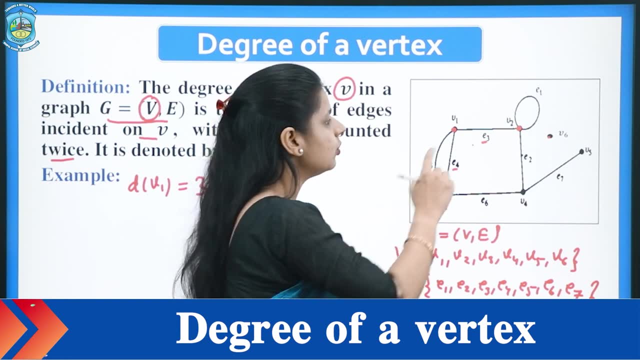 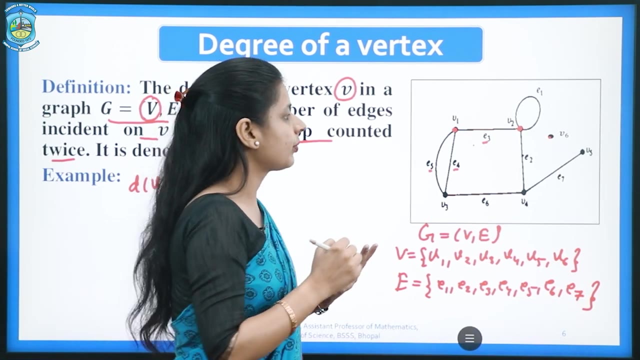 So the degree of this vertex V1.. When we calculate degree of this vertex V2, we have a self loop on V2.. That is, we have to count 2 for the degree and another 2 for these two incident edges, E2 and E3. 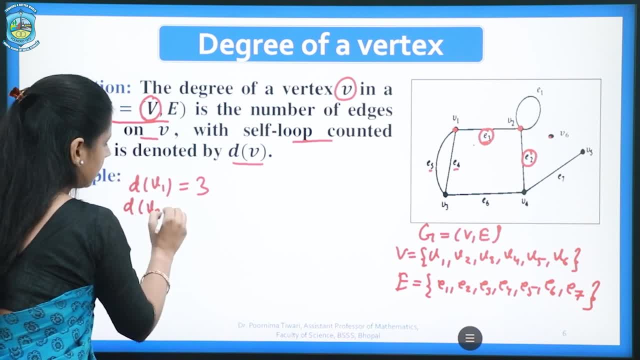 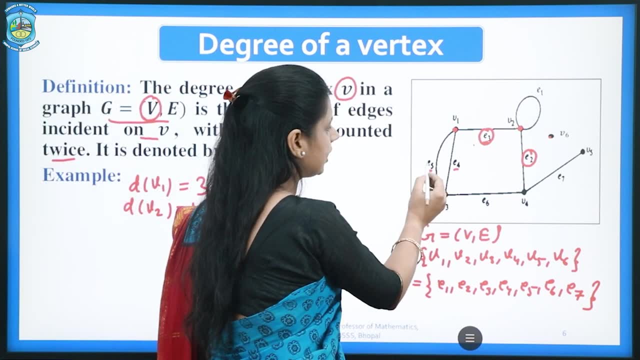 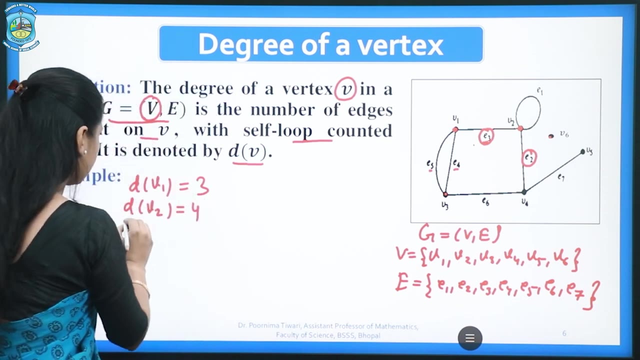 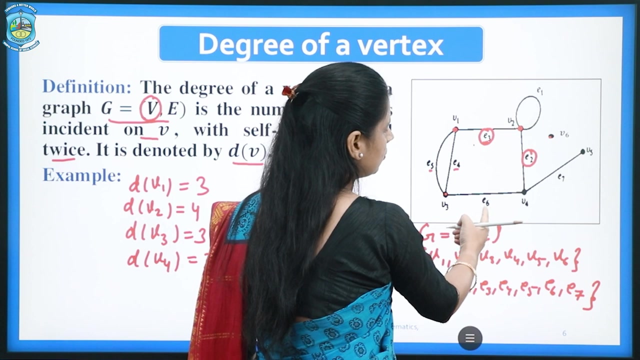 That is, degree of this vertex V2 is 4.. For the third vertex, V3, three edges incident on E8, E5, E4 and E6. So degree of this vertex V3 is 3.. Likewise, degree of V4 is also 3 because three edges- E2, E6, E7- incident on this vertex V4. 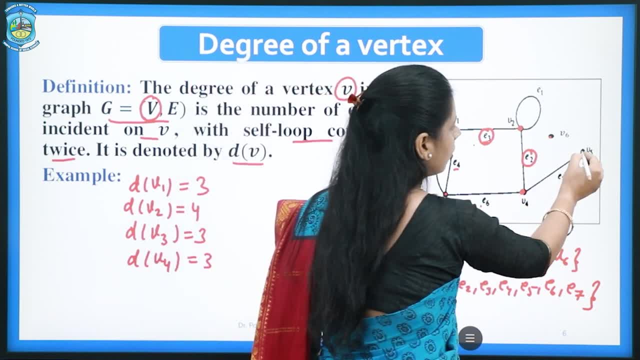 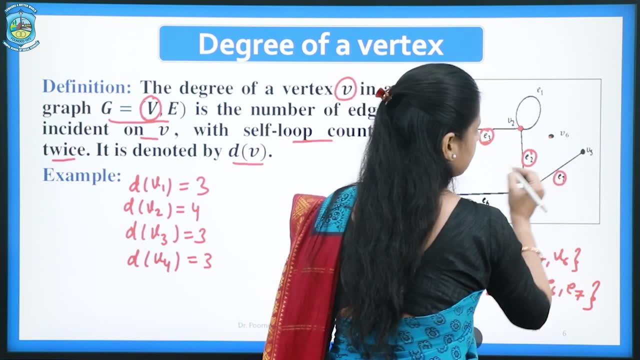 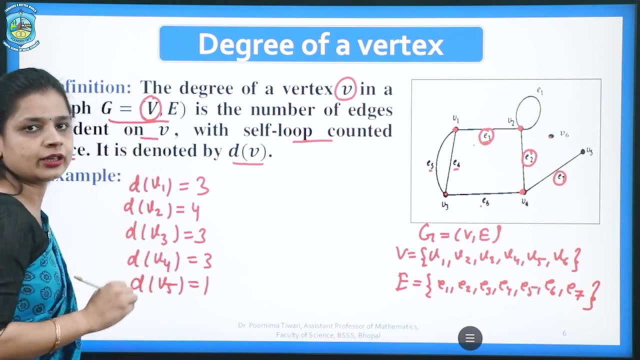 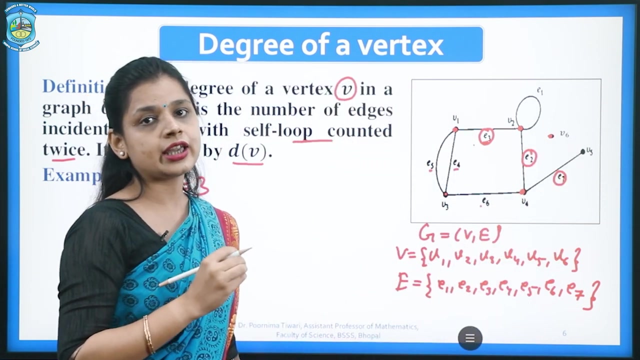 Next, we notice that on the vertex V5, only one edge incident on, which is E7. That is degree of this vertex. V5 is 1.. When we talk about this vertex V6, no edge incident on V6. That is degree of V6. 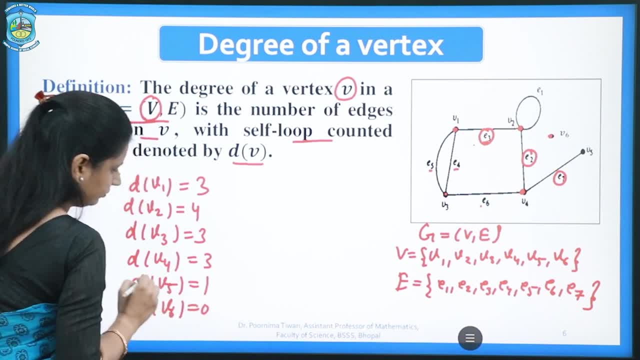 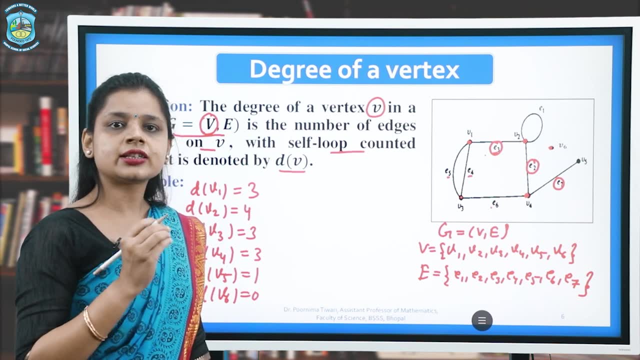 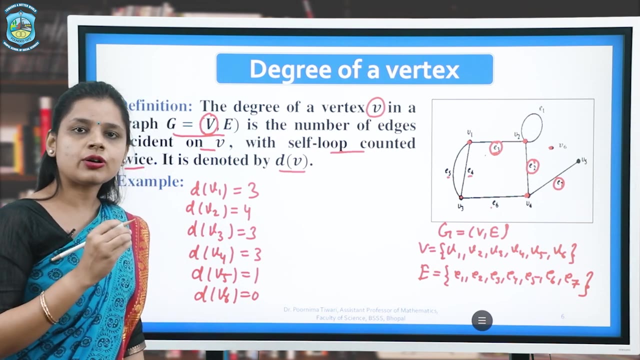 We can draw two relationships. vamos Now, if something is taken as 0 and V6 is 0. You must note down this fact: That if degree of a vertex is an odd number, vertex is called odd vertex, And if the degree of vertex is an even number, we call it as even vertex. 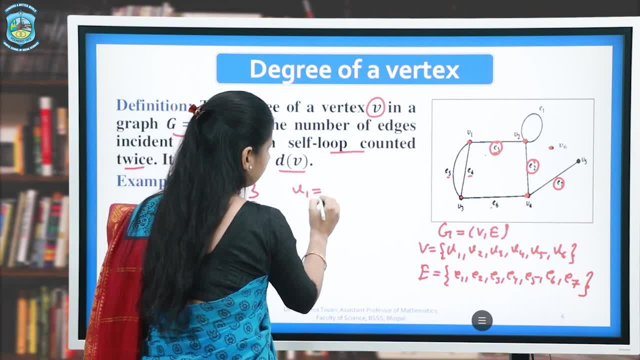 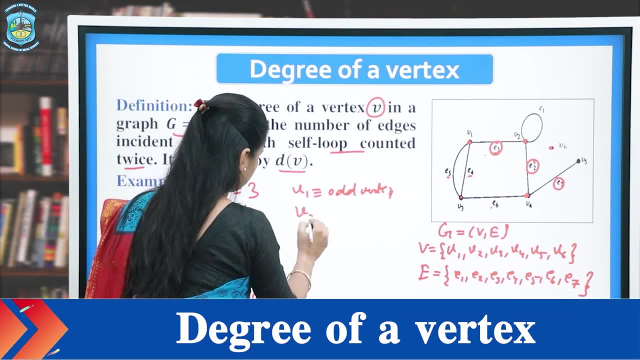 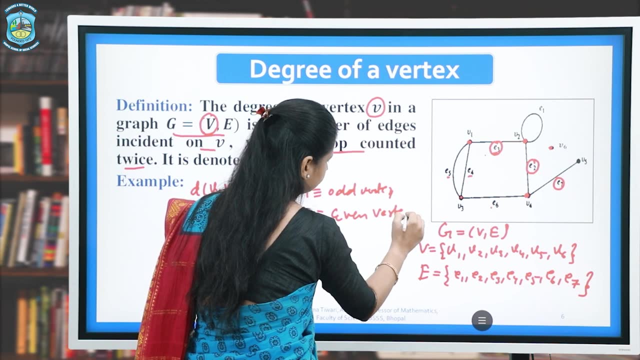 So degree of V1 is 3.. It means V1 is an odd vertex. Sorry, I overdrove a lot, Hurry, please write it down quickly. So how, according to this harus malu, Degree of V2 is 4, which is an even number. so V2 we may refer as even vertex. 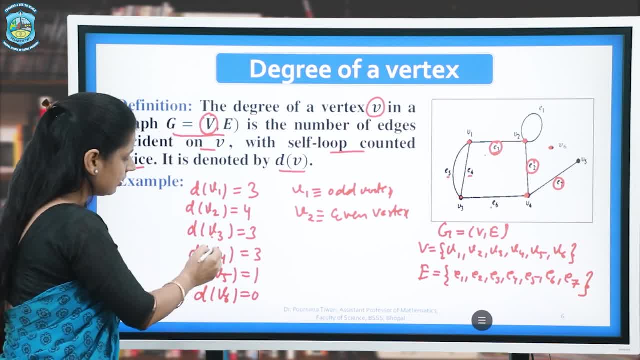 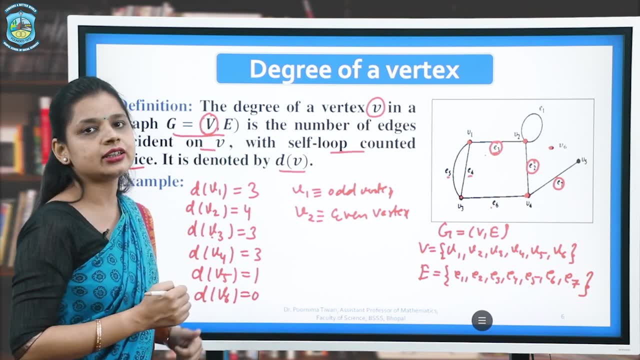 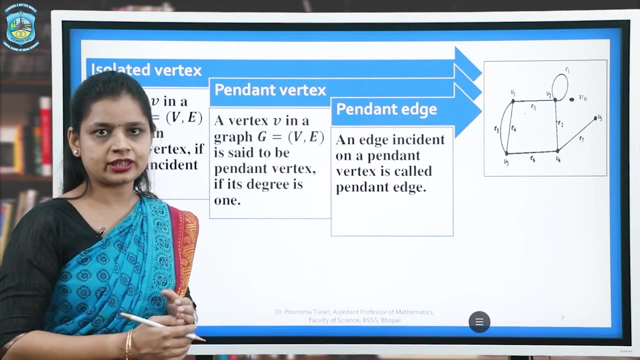 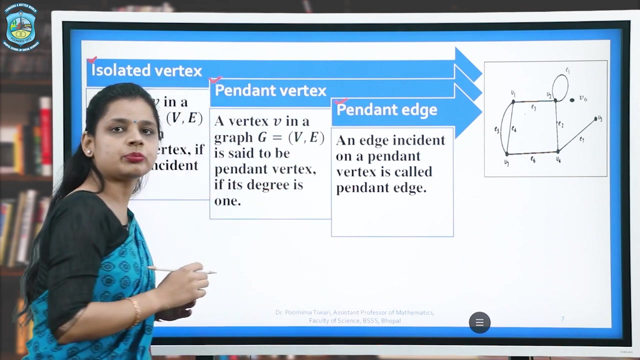 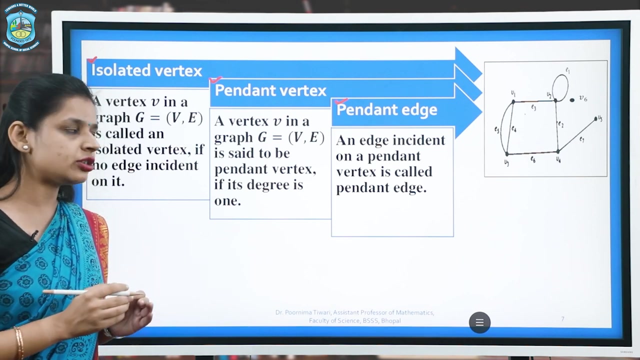 Likewise, V3 is odd vertex, V4 is odd vertex, V5 is odd vertex and V6 is an even vertex. This concept is associated with degree of a vertex, and here we have three definitions: isolated vertex, pendant vertex and pendant edge. A vertex V in a graph G is called an isolated vertex if no edge incident on it. 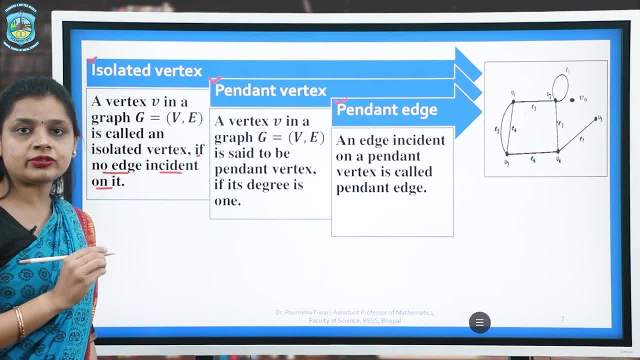 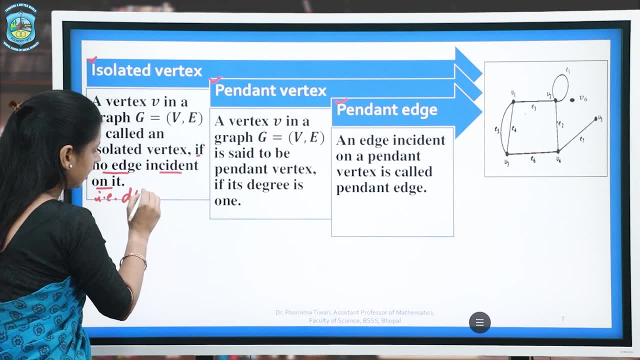 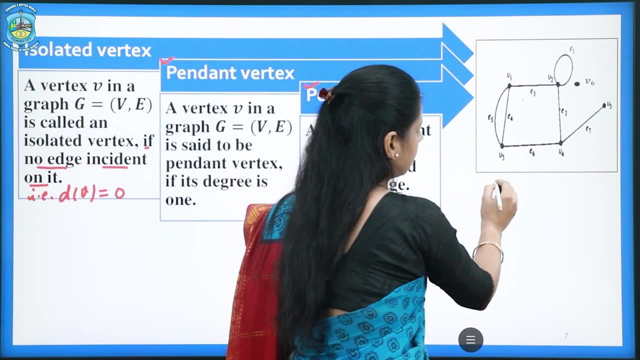 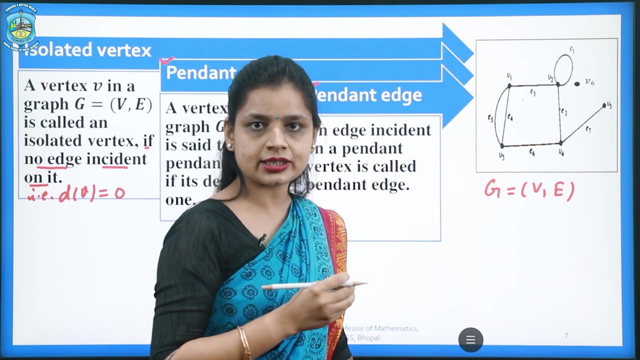 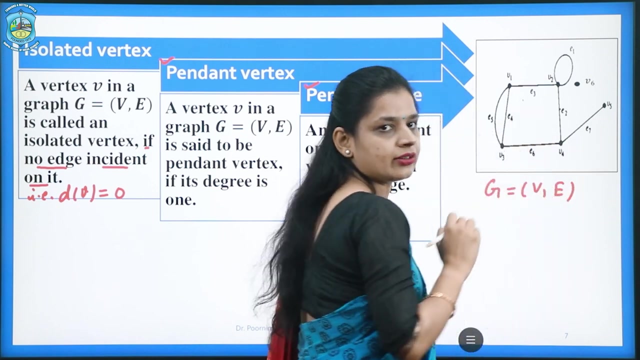 That is, vertex V is an isolated vertex if its degree is 0.. So we can write that is if degree of V is 0.. Now for the example. we will consider the same graph. G is equal to VE, where the set of vertices has six elements and set of edges have E1, E2, E3, E4,, E5, E6, E7.. 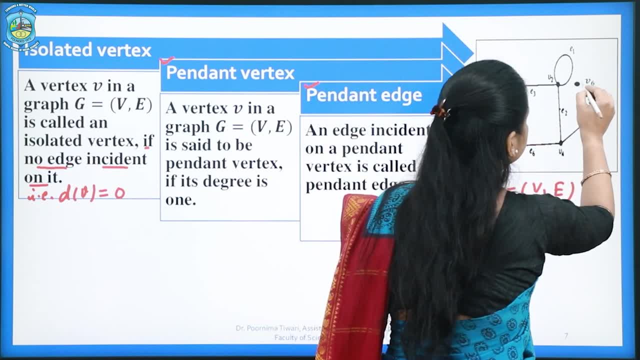 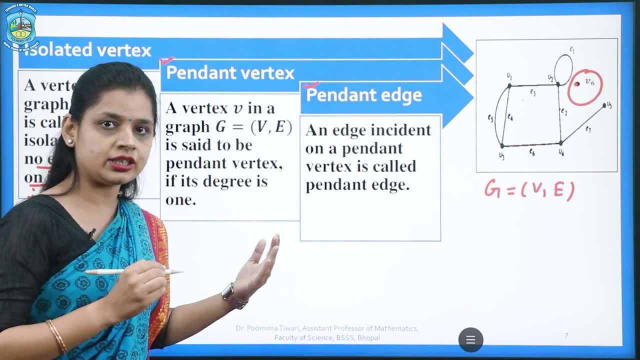 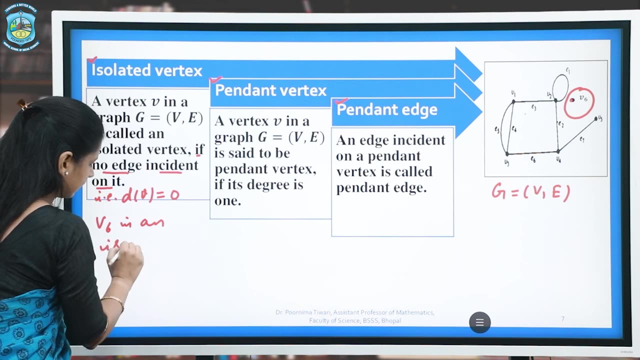 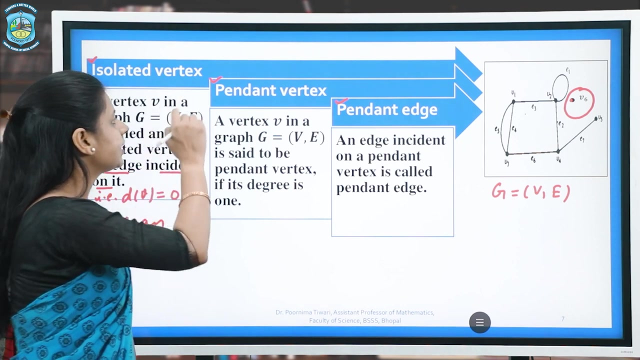 In the previous example we find that for this vertex V6, no edge incident on it. its degree is 0.. So in this graph, V6 is an isolated vertex. Next definition is about pendant vertex. A vertex is called a pendant vertex. 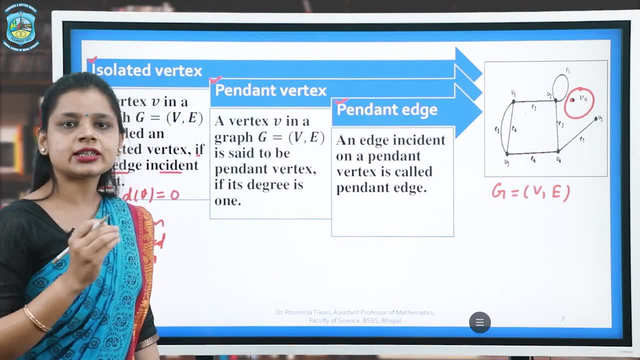 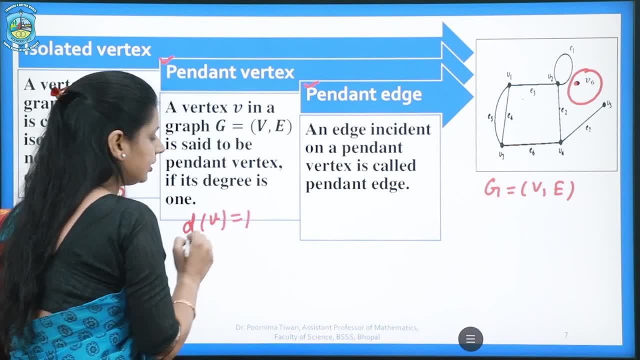 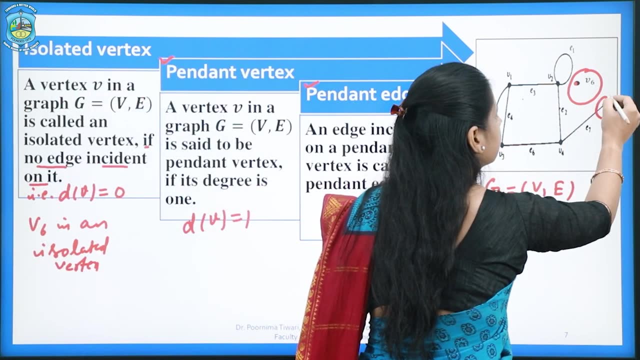 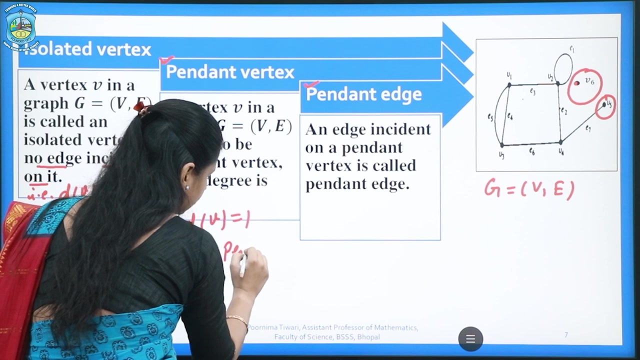 In a previous example we found that a vertex is called a pendant vertex if its degree is 1.. That is, if degree of V is 1, then this V will be a pendant vertex. In this graph we find that degree of this V5 is one, so V5 is pendant vertex in the given. 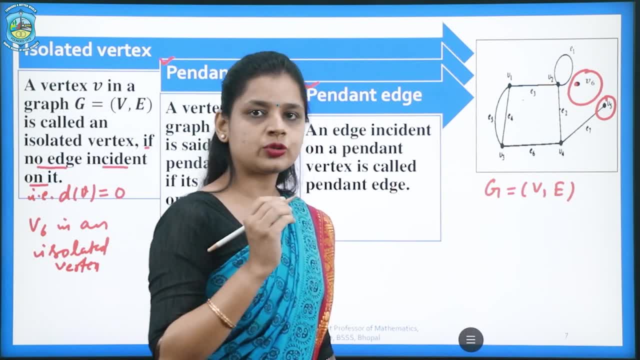 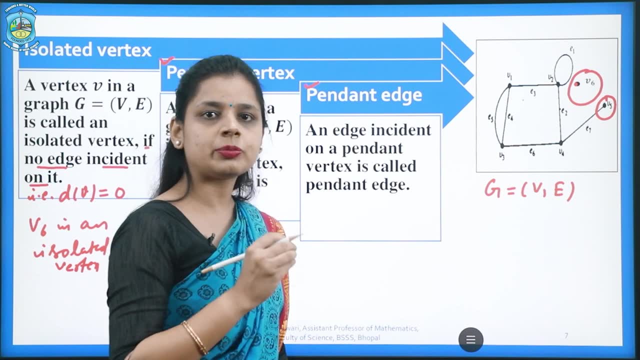 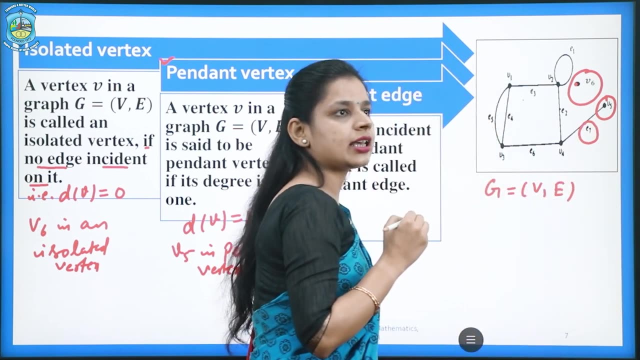 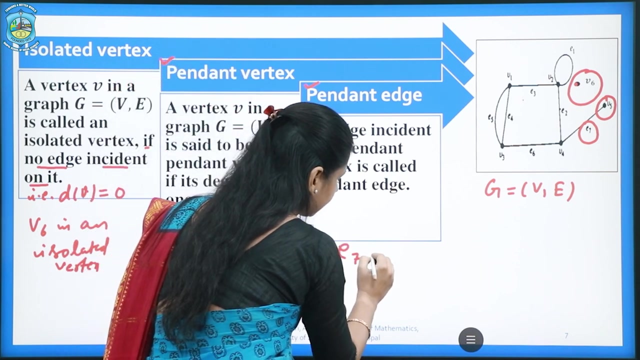 graph. Next definition is about pendant age, An age which incident on a pendant vertex is called pendant age. In the last example we saw that this age E7- incident on pendant vertex V5. So this age, E7, is a pendant age. 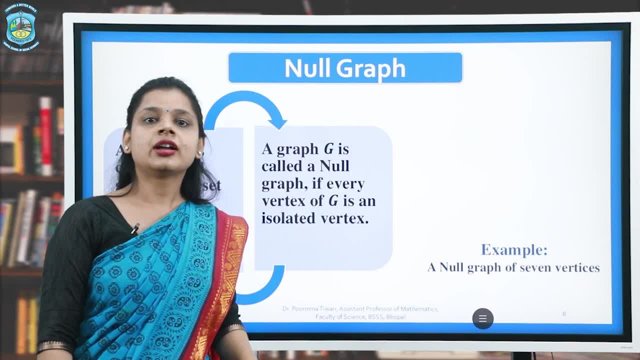 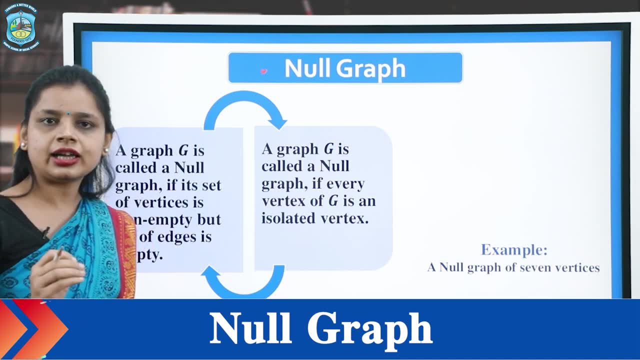 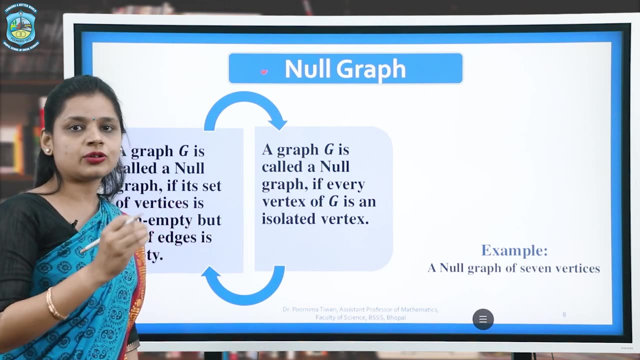 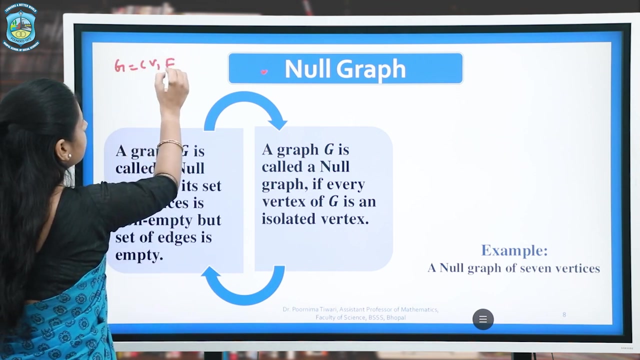 Next definition is about null graph. A graph is called a null graph if its set of vertices is non-empty, but its set of edges is empty. That is, we have this graph: G is equal to VE, such that the set of vertices is non-empty. 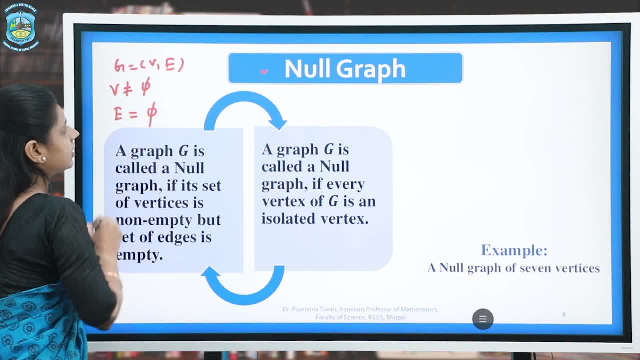 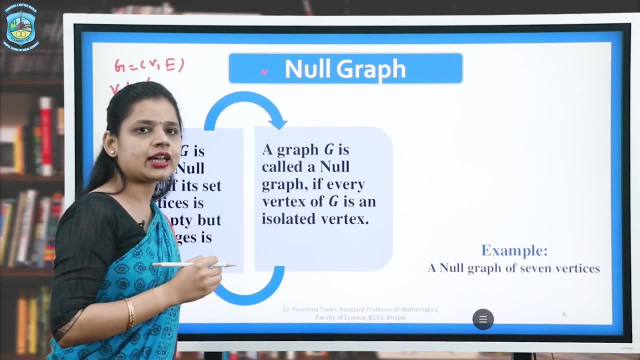 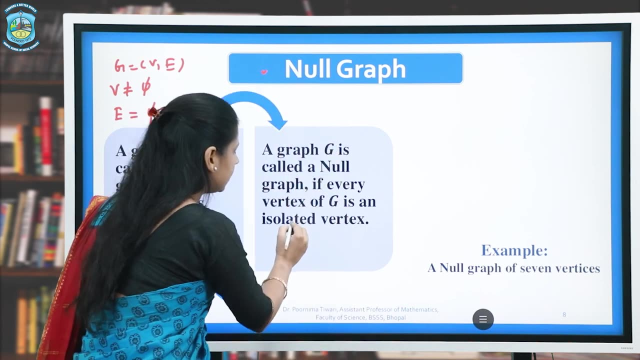 and the set of edges is non-empty. So this is a null graph And set of edges E is empty. Then we call this graph G as a null graph. Or we can say that a graph G is a null graph if every vertex of G is an isolated vertex.